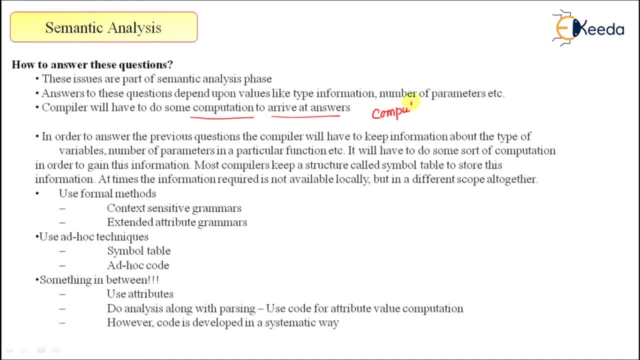 earlier that it has to perform some computation. there is some level, some type of computation required. okay, so in order to answer this, uh, this previous question, the compiler have to keep track information about the type of variable. few things it has to keep track, and among them the first: 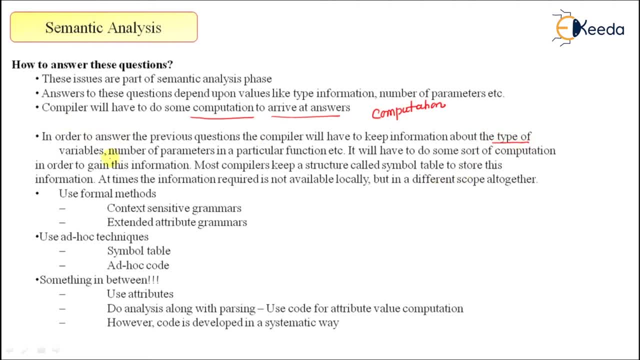 thing is the, there's the, it has to keep track of the type of the variable, uh, number of parameter in a particular function, etc. and it will have to do some sort of computation. okay, so, as the statement, as i said earlier, in order to gain this information. so something has to be, you know, done. 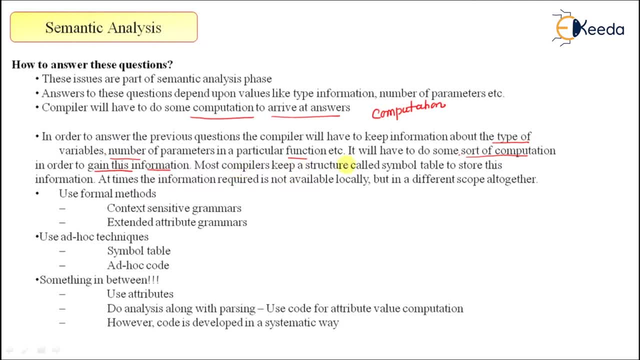 again, to, to, to perform this, to again this information. most compiler keep a structure called symbol table- okay, so that i told you in the beginning symbol table to store this information and at times information required uh is not available locally and but in different scope together altogether. so sometimes you, you may need to require to access other, other places or other, let's say, function to. 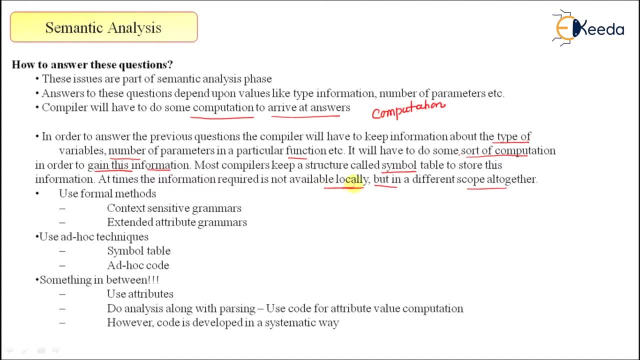 get the information uh related, so not available locally, means that a different scope- and it can be a different uh different scope means it can be a different function. all together, okay, so the the question is: we have to perform some that, that the challenge, that we need to perform some computation and the only thing is 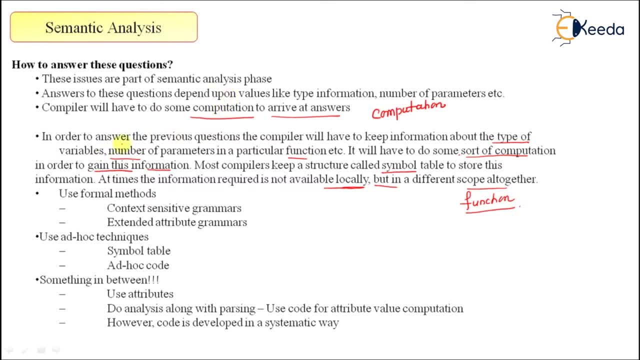 that how we are going to do this thing, okay, so there are few solutions. are there related with this? that one is your context sensitive grammar- okay, so that that is one of the solution. that context sensitive grammar or extended attributed grammar- okay, now this is the new term- extended attributed grammar- okay, symbol. 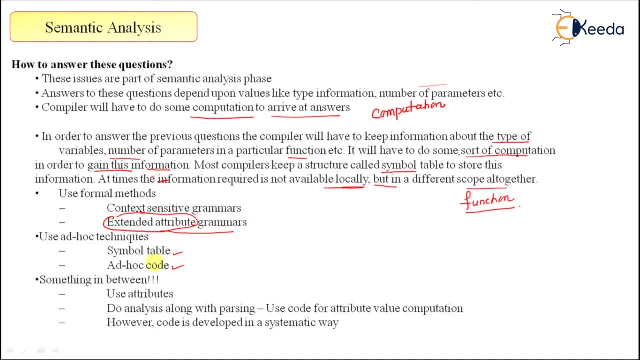 table is a way to store all the information you can compute and store and something in between, that that uses attribute and do analysis along the parsing. use the code and attribute for the value of computation- okay, but in a systematic way. so now, or something in between, that is, that is you we will use. 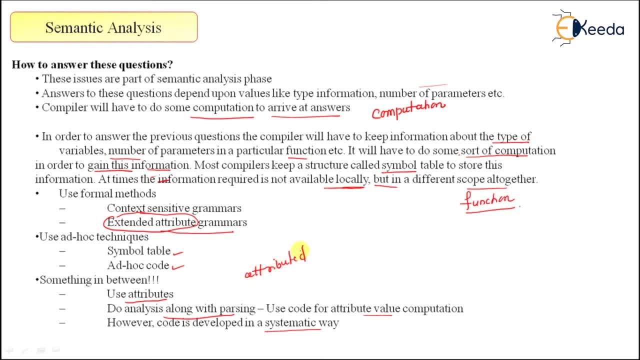 now attributed grammar: a tree, put it grammar. now you generally general term is: arrive here. what exactly an attribute? okay, so what is an attribute? so suppose I give you an object? okay, I'll give you object. let's say, I'll give you a table, okay, so now there is some characteristics. are 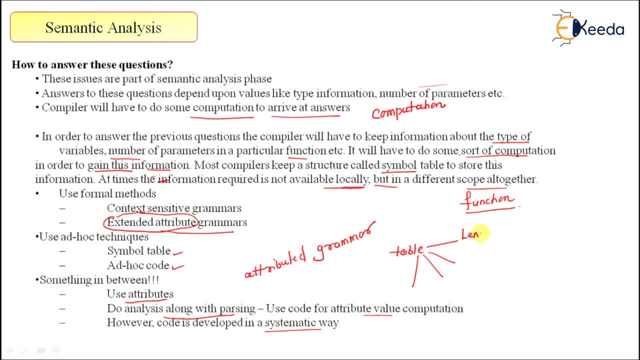 there which defines this table. okay, the length: okay, length is an attribute of the table. the weight is an attribute of the table. the height: okay, it's your height- can be an attribute of the table. the color can be the attribute. get also attribute. that will define a. depends upon the object. 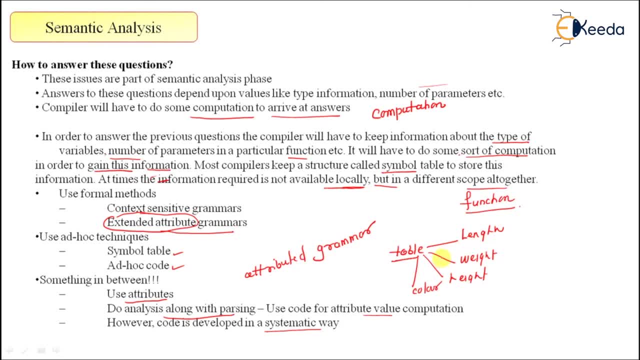 okay, it depends upon the object and it defines its few characteristic. okay, so that basically is called an attribute. now to explain you, the- you know this I have already spoke- means previous in this session I spoke talk about a few this, this, technical terms, technical terms. now here i'll give you one informal, um, informal, let's say. 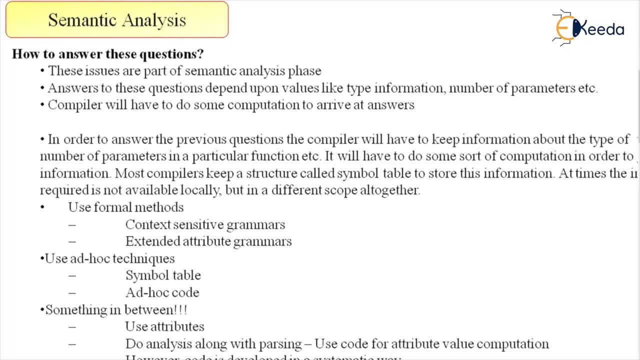 informal way of- okay, informal way of you know or understanding this particular topic, and suppose i'll say: baby is crying. okay, now, this is the statement: that baby is crying. okay. so now here, what syntax analysis analysis phase does, is it only find out whether this baby is crying? is a correct sentence or not? okay, correct. correct statement or not correct. 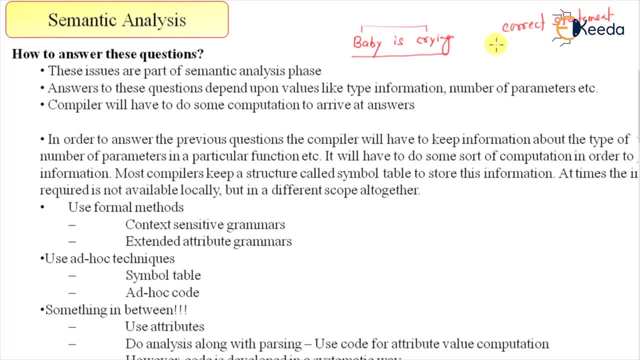 string or not, it's a correct statement or not. now, what i'm more interested here in this case is is understanding a meaning, and what is the meaning is that there is a small child, there is a small child is, and that child is intra in, is, is is having some issue or is is crying. let's say the same. 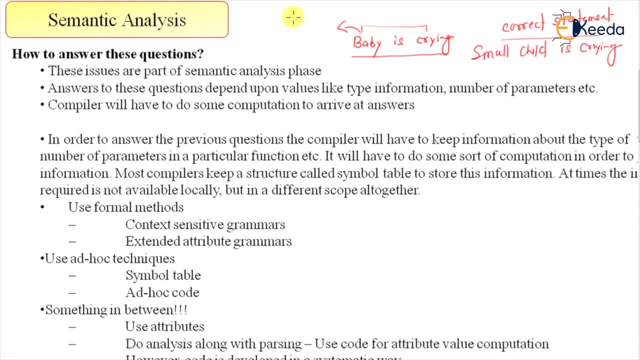 statement. there's a crying, so i know that is a baby. baby will have a. you know she's a small. the age, the year, mayor of female, that can be the attribute. and crying is also carrying some meaning: that she needs something, she is in, she is, she is hungry or something like that. okay, so now.